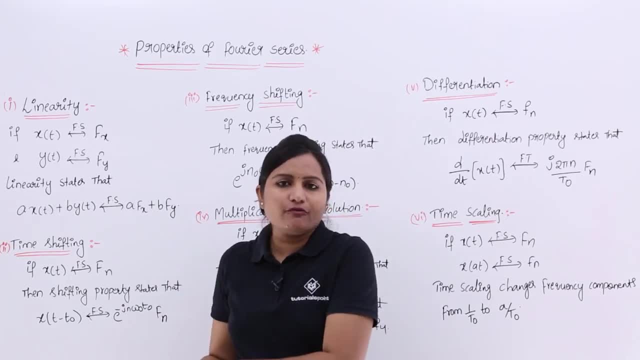 can take the same signal. If you changed that signal, then what is the change of Fourier series coefficient that we want to discuss here? Properties means what we are going to discuss means, For example, Fourier signal. if you are having a particular Fourier series. 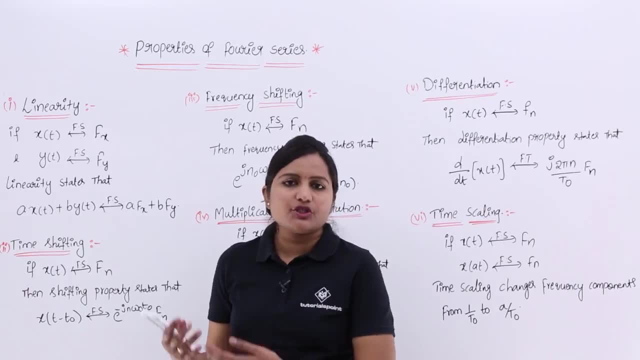 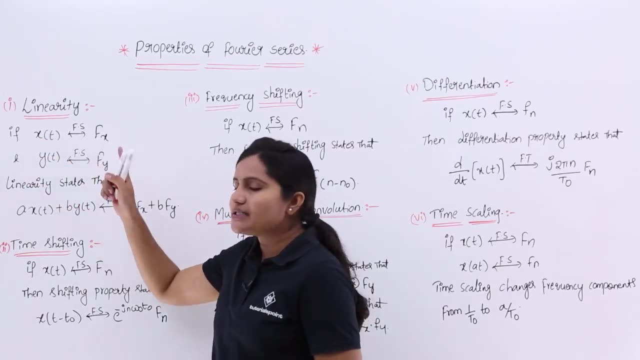 coefficient. if you changed the signal, what is the effect of that change on the Fourier series coefficient that we are going to discuss here? For example, Fourier signal Xf, t, if you consider Fourier series coefficient as effects, as I already told you. So suffix. 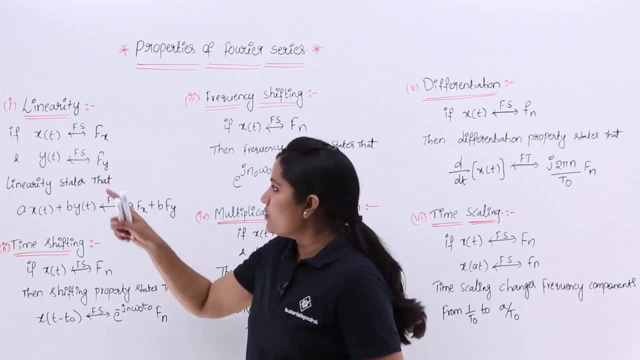 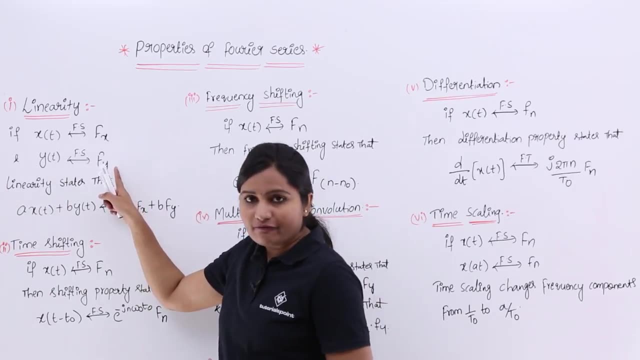 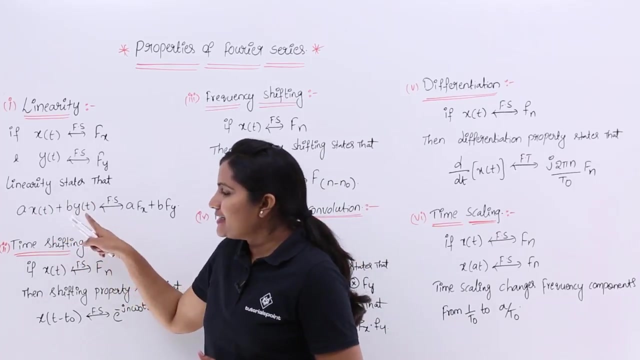 or naming of Fourier series coefficient is your wish. So here, if X of t has Fourier series coefficient f- x and Y of t signal is having Fourier series coefficient f- y, like this: if you consider, then linearity property states that. So if you added these signals, 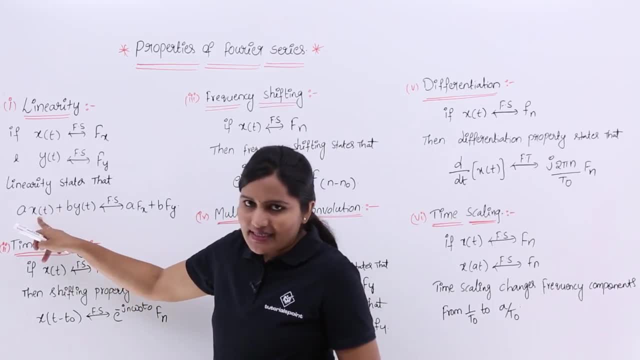 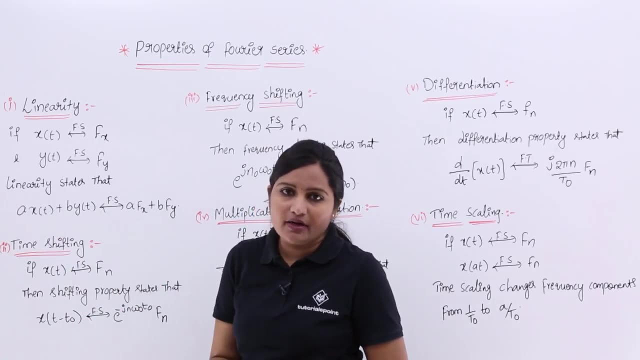 by scaling like this. So you, if you scaled X of t and Y of t with different scaling coefficients, and if you added and if you make as a different signal from X of t and Y of t, then for that resultant signal, So this added signal is also a signal. why? because you are just scaling. 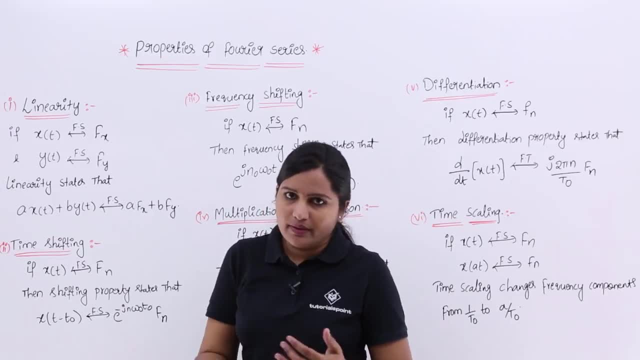 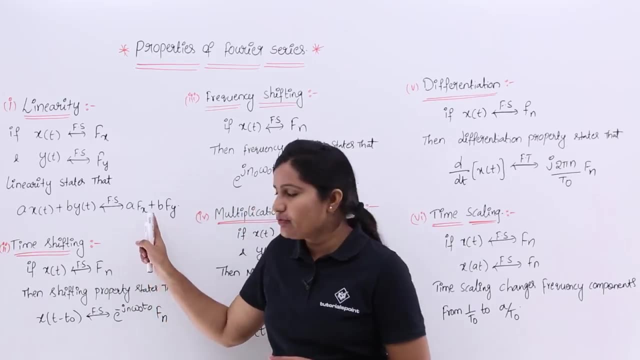 and adding two signals, the resultant is also may be a signal, that signal for that signal. if you want to represent in Fourier series, the series coefficient you need to consider is also follows: same condition: A f x plus B f y, So x, X of t having f x and Y of t having f y. So if you are adding signals like this, the 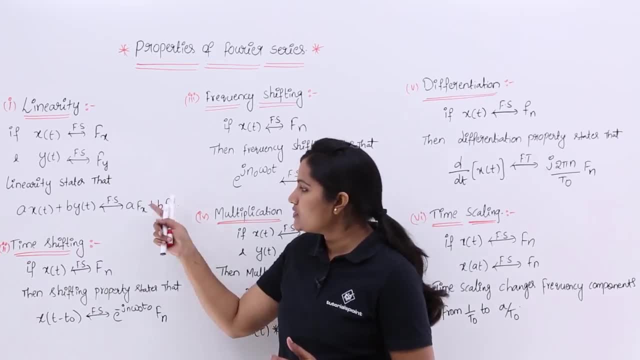 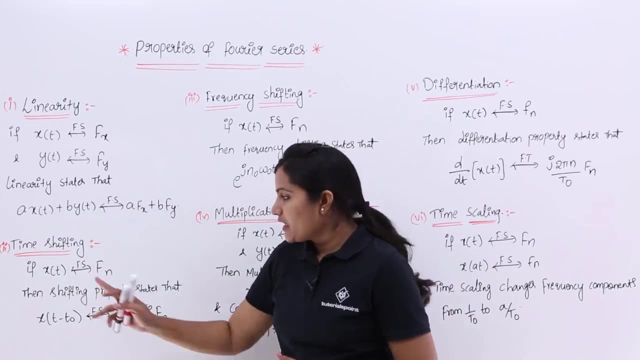 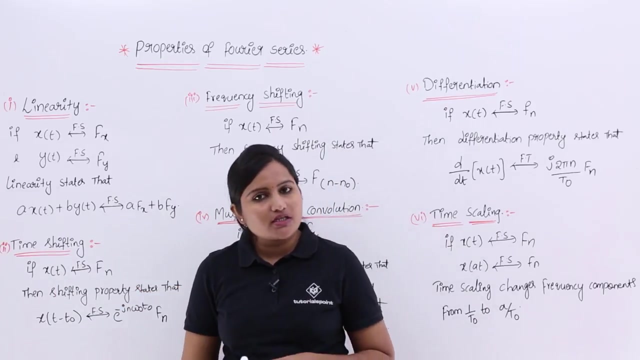 Fourier series coefficient value you can take also vary according to that only. So this is about linearity property. Coming to time shifting property, if X of t having Fourier series coefficient, f n- this time I am considering f n- So if X of t is having Fourier coefficient, 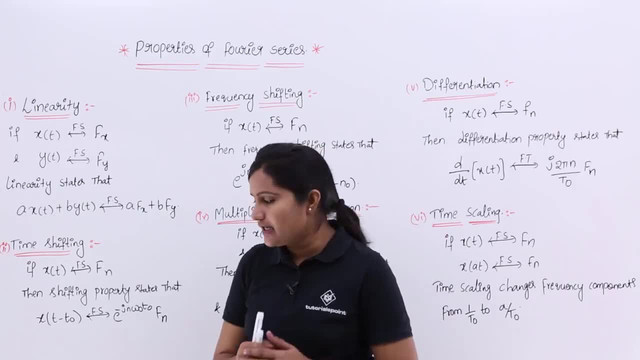 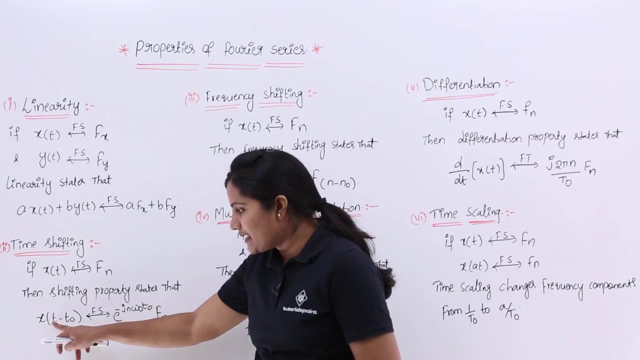 f, n, and then shifting property states that if you consider shifting property then you change the time shifting of the signal. So as we are considering time shifting property, So it states: when you changed the signal by shifting the time, then Fourier series coefficient is multiplied by e power minus j, n, omega, naught, t naught. So here you can see you are having 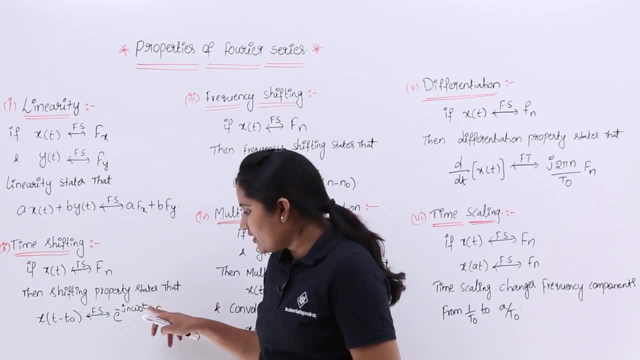 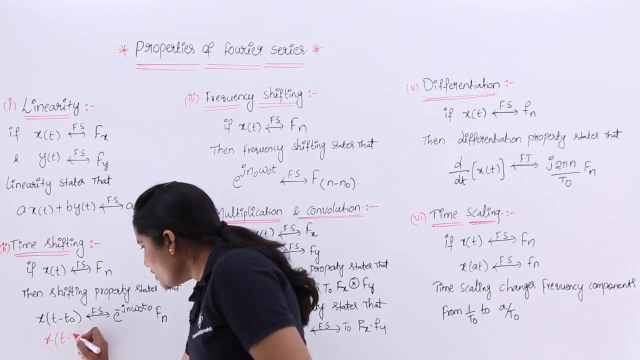 X of t plus t naught. So e power, j n, omega naught, t naught will be there. for example, if you are changing, you are shifting t minus 2. So for this you can take as time shifting property and you can take it as time shifting property. So you are taking x of t plus t. 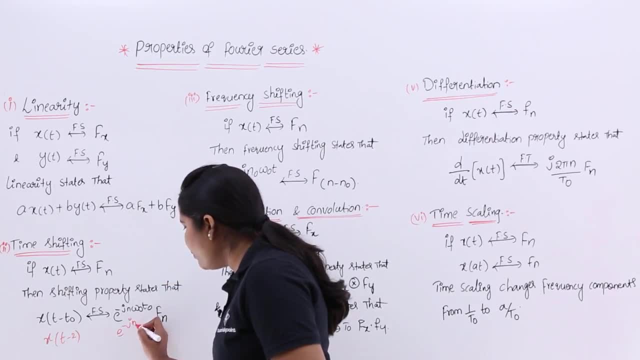 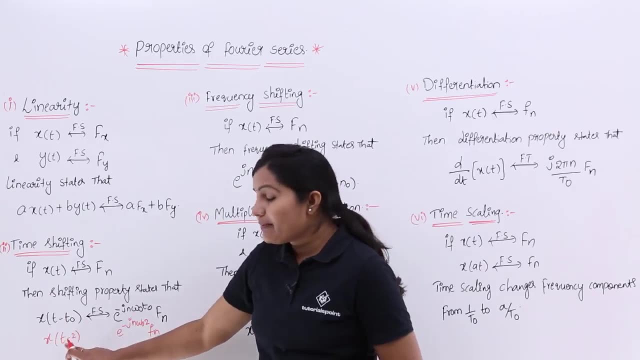 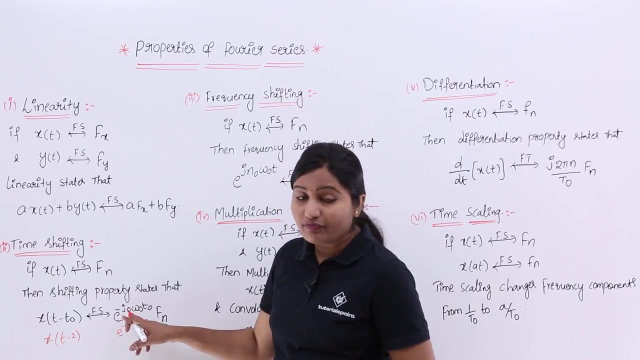 then you are getting e power minus jn, omega naught to fn. So like this you are getting, So like this, the change will be there. For example, if you are having plus value here, that means if you are having plus t naught- then you can say: this is Fourier series quotient. 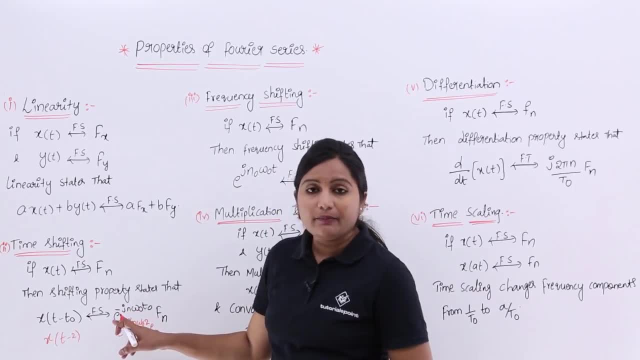 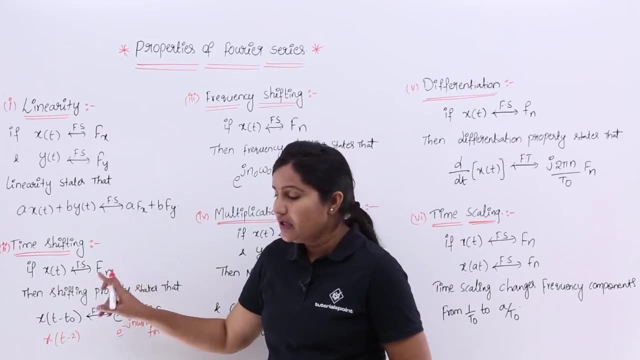 that you need to consider will be changed with multiplication factor with positive e power. That means if you are having x of t quotient as fn, then if you want Fourier series quotient for x of t plus t naught, then you need to consider this as e power, jn omega. 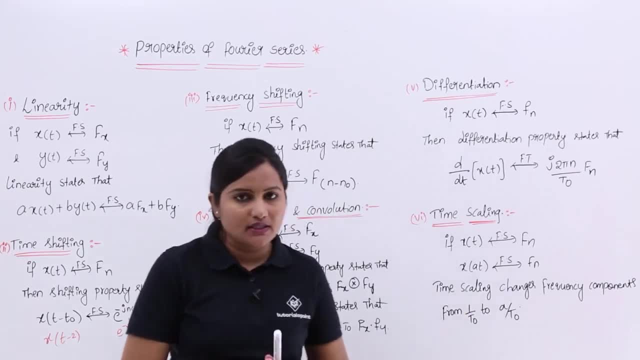 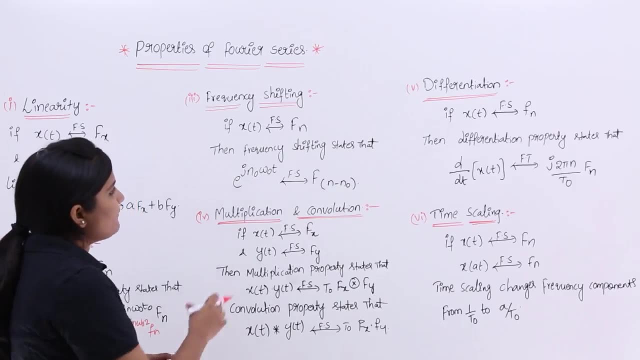 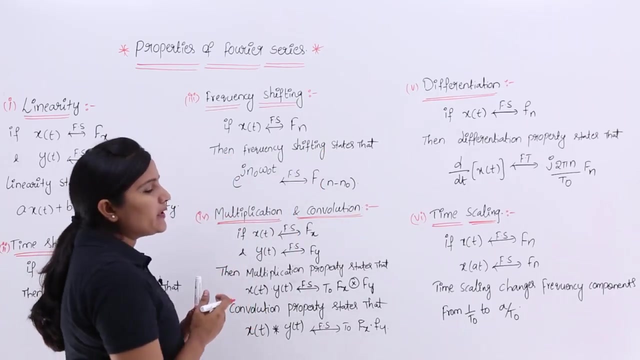 naught t, naught fn. So this is time shifting property. So coming to frequency shifting property if x of t Fourier series quotient fn. if you consider the Fourier series quotient for x of t is fn, then frequency. So this shifting property states that e power jn naught omega, naught t into x of t. 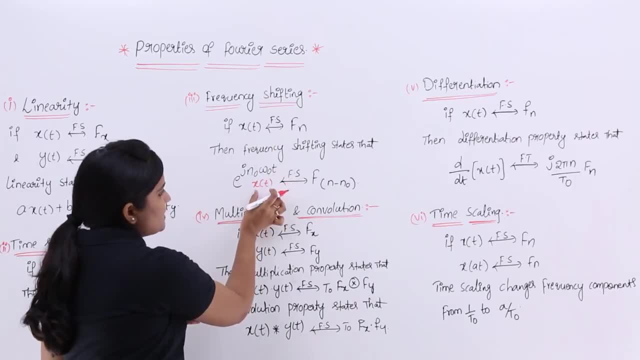 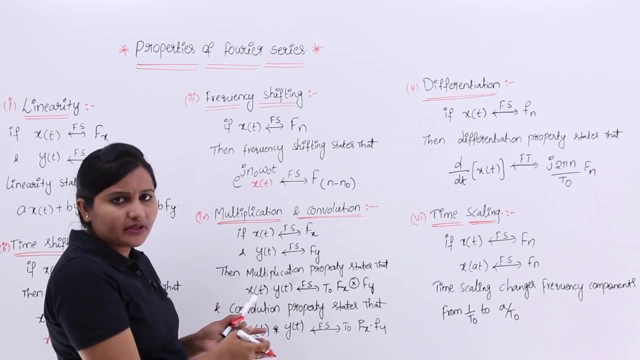 signal. that means this signal, this x of t signal. if multiplied with any exponential, that means any other signal, any other frequency signal is nothing but any other frequency. then that frequency is having effect on coefficient of this signal, like f of n minus n naught. So here you can see that is going to subtract. 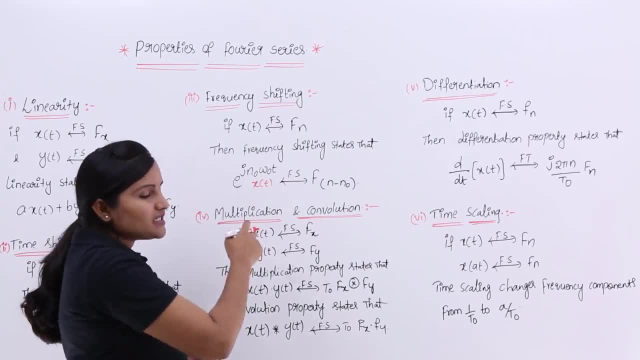 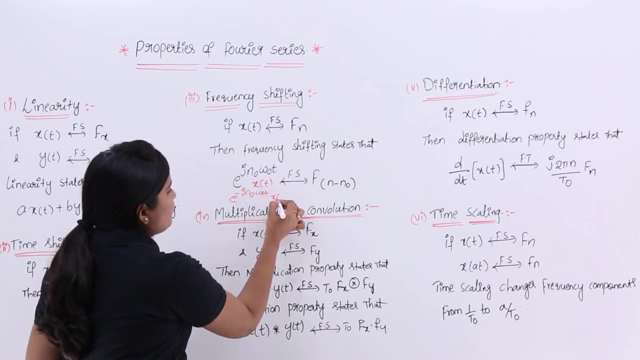 For example, if you are multiplying e power minus jn, omega, naught, t, that means if you are multiplying e power minus jn, naught, omega naught, t, x of t, then you need to consider the Fourier series quotient as f of n plus n naught. Just keep in mind when you are having plus here you 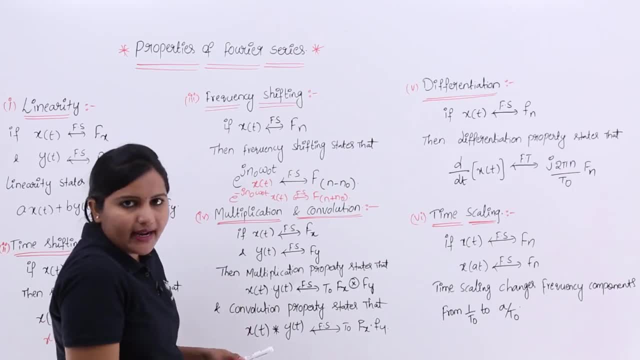 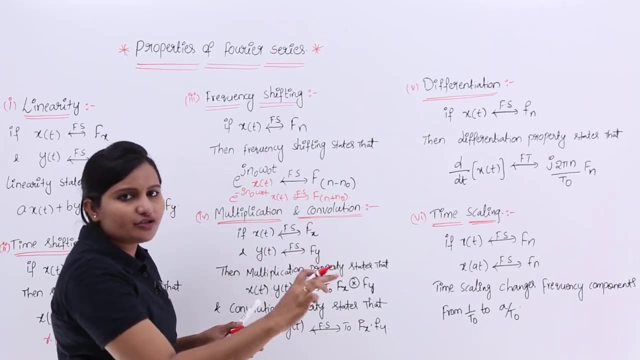 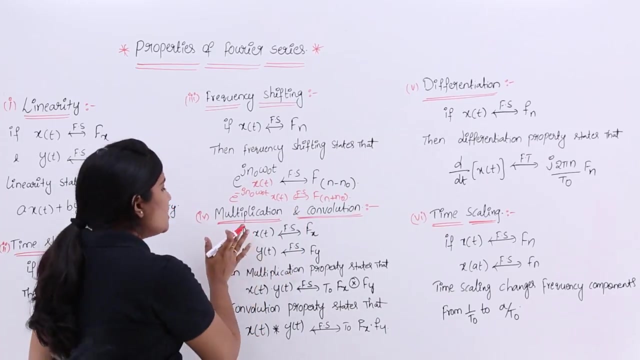 need to differentiate, that means you need to subtract whatever signal is there that you need to subtract. So here, that means from actual frequency you need to subtract. So here, multiplication and convolution property. next property is multiplication and convolution. So if x of t having Fourier series quotient f, x and y of t is having Fourier series quotient, 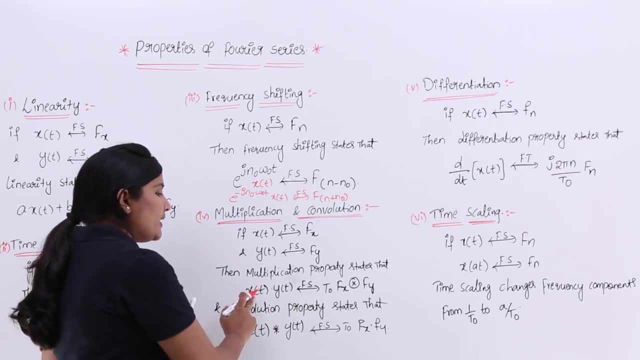 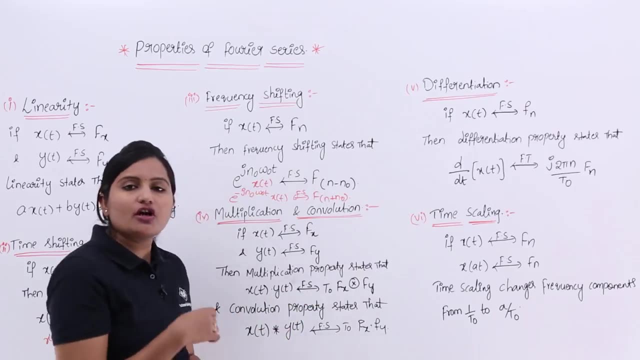 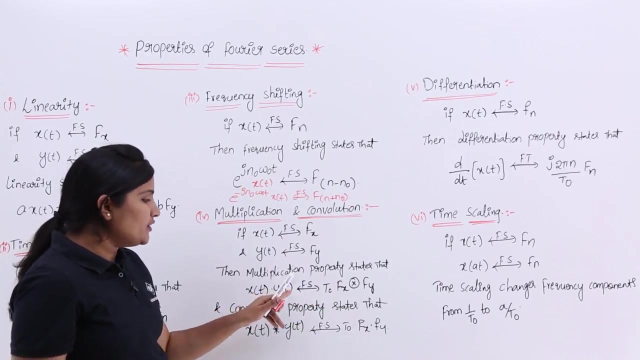 f, y. then multiplication property states that multiplication of these two signal, for multiplication of these two signals you need to consider convolution of coefficients with a. with a coefficient, That means convolution of Fourier series coefficient, So you may get some coefficient value also here. So that is I am going to represent with t naught here, So x of t into 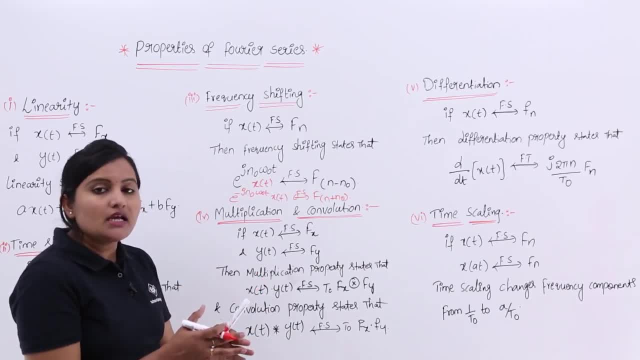 y of t, if you consider multiplication of two signals, So then for that resultant signal, the Fourier series quotient that you need to consider is the convolution of actual coefficients. So, in the similar way, if you want convolution of two signals, if you want the coefficient, 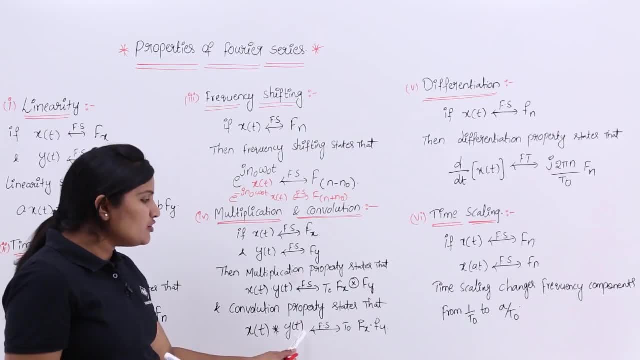 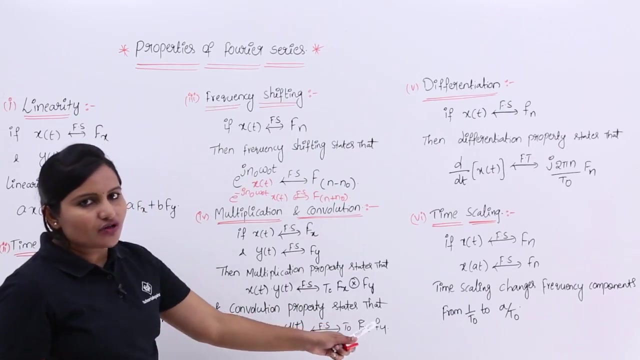 of Fourier series to represent convulsion of these two signals. then Fourier series quotient you need to consider in multiplication. If you want multiplication of signals, you need to consider convolution of quotients. If you want convolution of signals, you need to consider multiplication of quotients. So 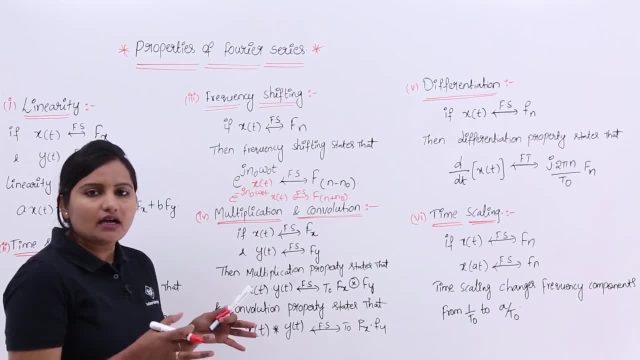 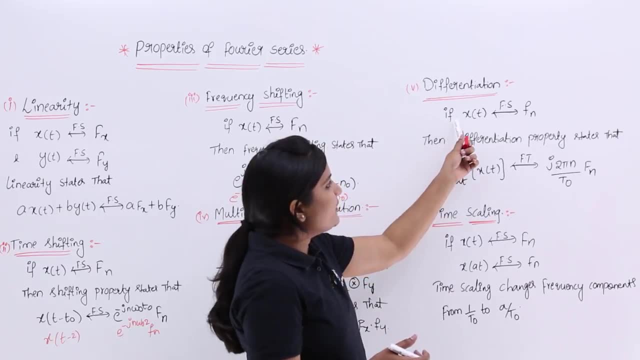 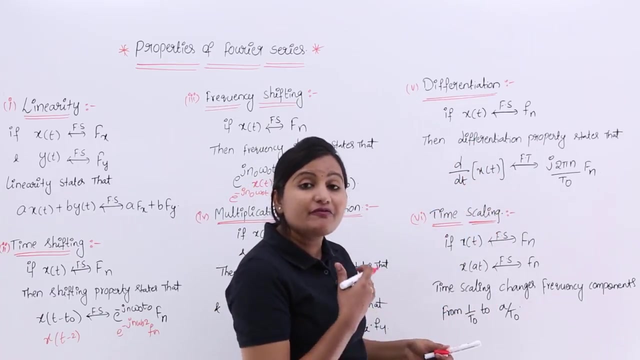 here t naught indicates any multiplication factor occur during that process. So, here differentiation property. Next property is differentiation property differentiation. �� So, if XRT Fourier series coefficient f n if you consider then differentiation property states that if you differentiate this d by dt of XRT if you differentiate your signal 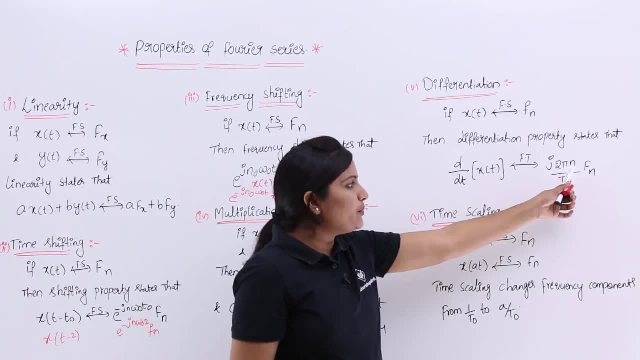 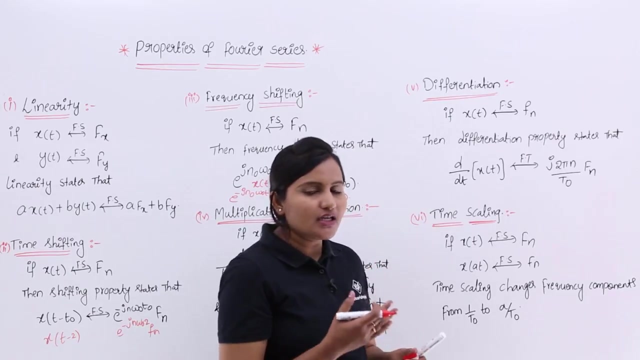 then Fourier series will change like j, 2, pi, n by t naught, f n. So finally you are having time scaling property. So if XRT Fourier series coefficient f n, if you scale time also, you are having same signal. So that is why Fourier series quotient is not going to change. 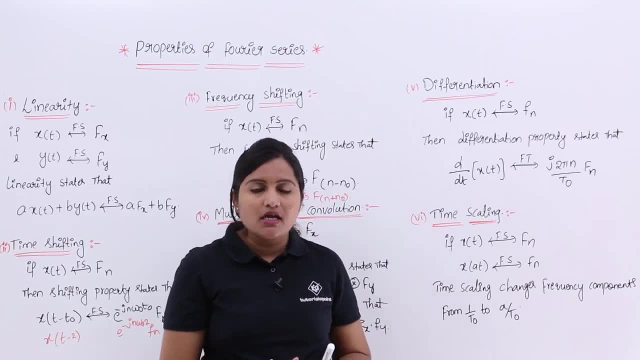 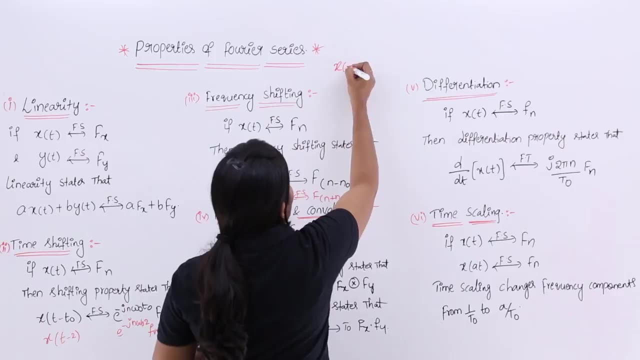 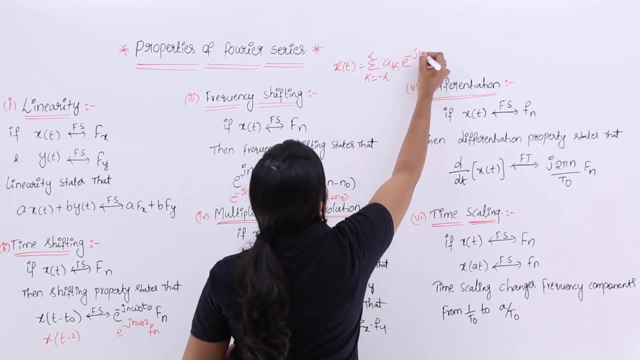 but it will changes the frequency components. So in the starting classes itself we discussed that. So we are going to represent any signal, XRT in terms of Fourier series. as k is equivalent to minus infinity, to infinity, ak into e power jk. omega naught t, So plus jk. So this is: 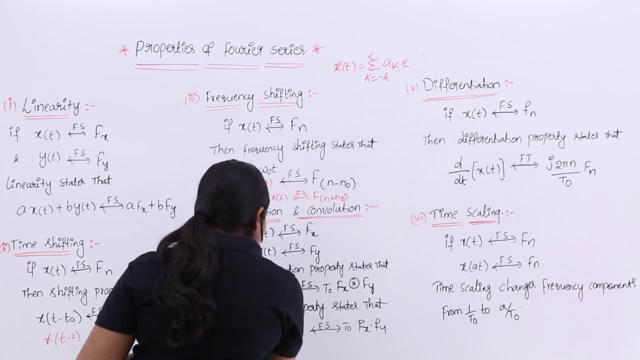 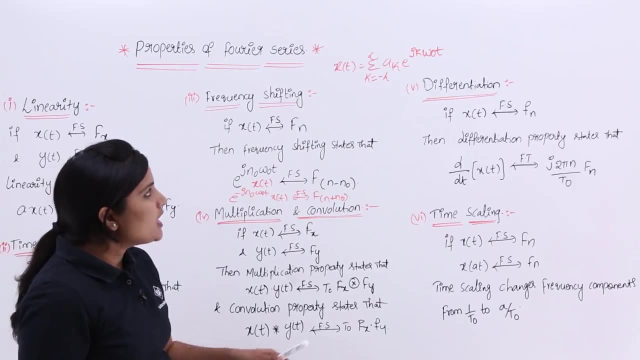 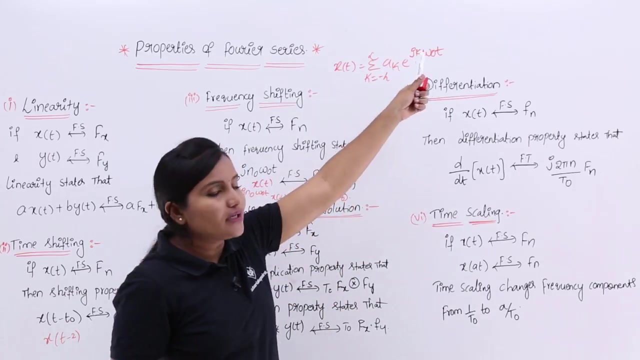 plus jk omega naught t. So e power, jk omega naught t. So like this we are representing any signal in Fourier series. If you consider this omega naught here, this is the fundamental frequency. That means if k is equivalent to 1, that is omega naught. So if the term for k is equivalent to 0, is 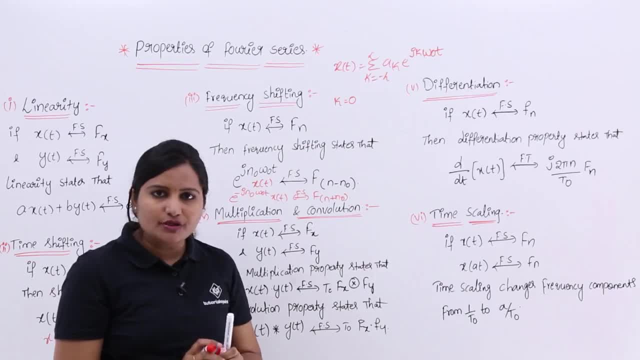 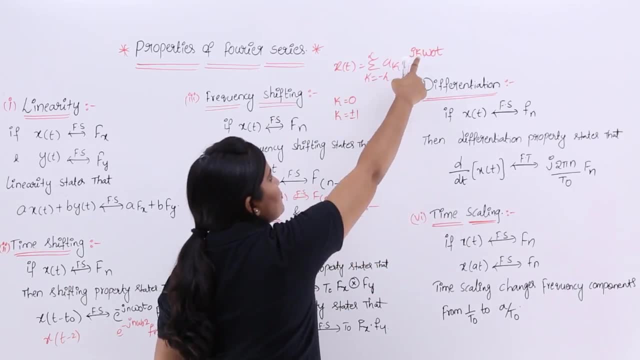 called as a constant. The term for k is equal to 0. is a constant. The term for k is equivalent to plus or minus 1.. If you consider k is equivalent to plus or minus 1.. So if you consider k is equivalent to plus 1 or minus 1.. So omega naught value, you are having only omega naught. 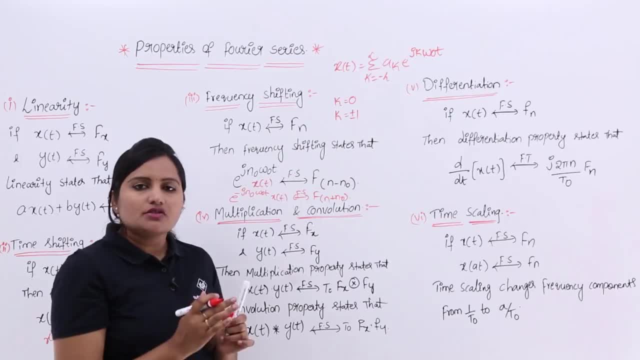 there In the e power you are having only omega naught, So there is no multiplication factor for that fundamental frequency. Then when k is equivalent to plus or minus 1, then that is called as fundamental components or first harmonics, That frequency components. 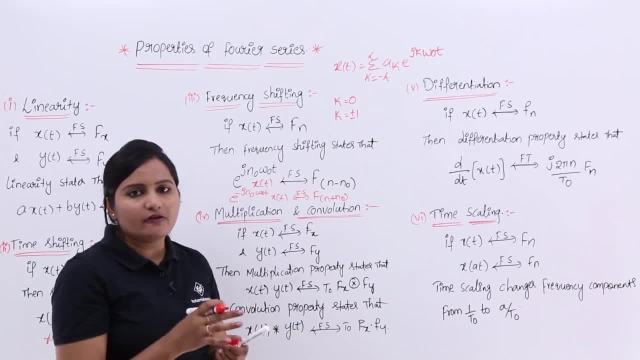 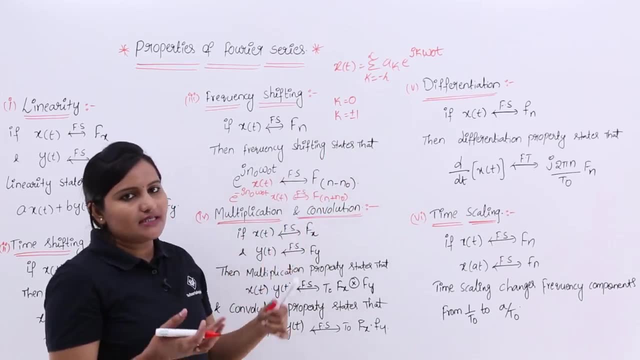 in that signal are called as fundamental components or first harmonics. When k is equal to 1, then that is called as fundamental components or first harmonics. When you ask to find out the fundamental components or first harmonics, you need to substitute: k is equivalent to. 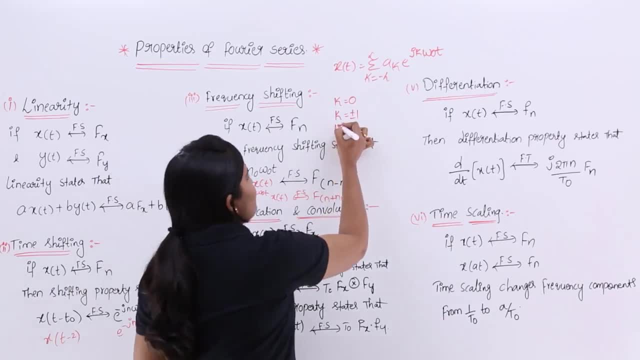 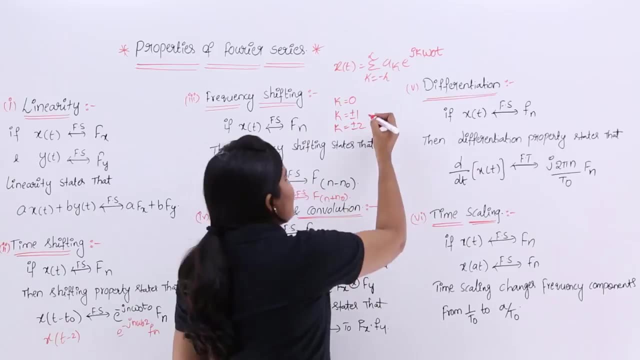 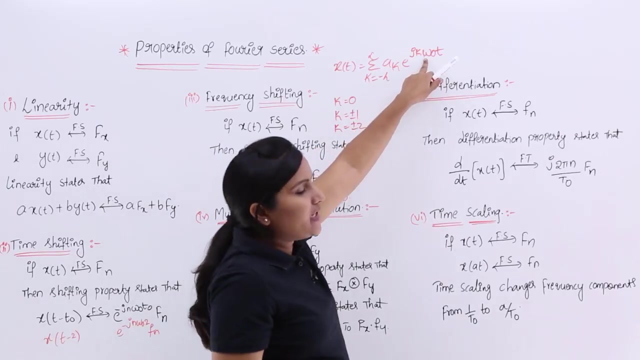 plus or minus 1. So if k is equivalent to plus or minus 2. So second harmonics: plus or minus 3.. So third harmonics like that, plus or minus n, you will get nth harmonics of that frequency. So now here these are called as frequency components, where omega: 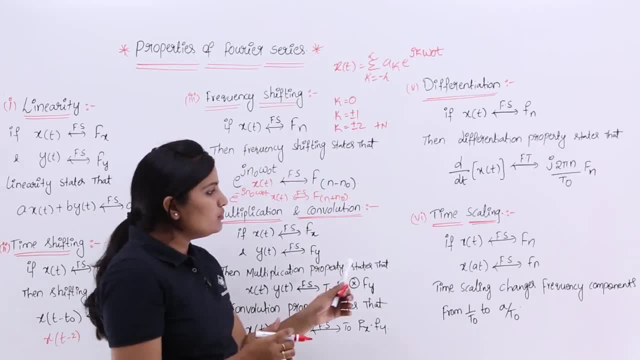 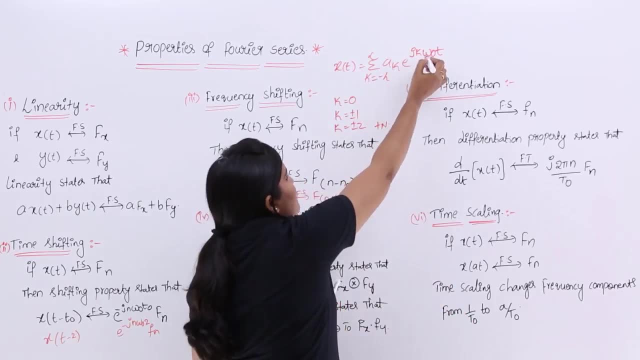 naught is equivalent to 2 pi by capital T. So you know that k is equivalent to 1.. So you know that. So fundamental time period is 2 pi by T. that relates this omega naught. that means omega naught is equivalent to 2 pi by T or T naught, you can consider It will. 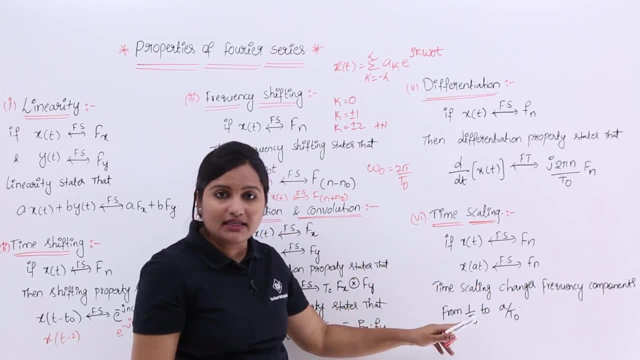 changes the frequency component. If you scale the signal, it is not going to change. the Fourier series quotient is not going to change, but the frequency components are going to change from 1 by T naught to a by T naught. This scaling will not change. So you know that. 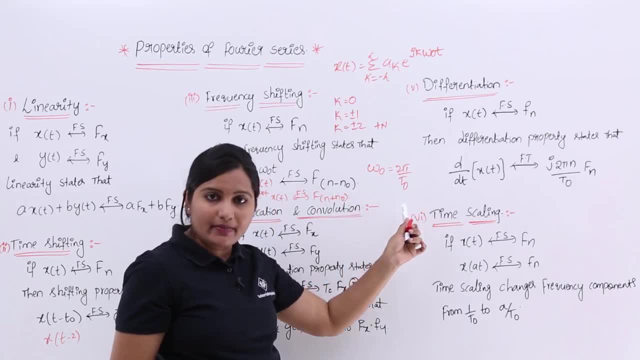 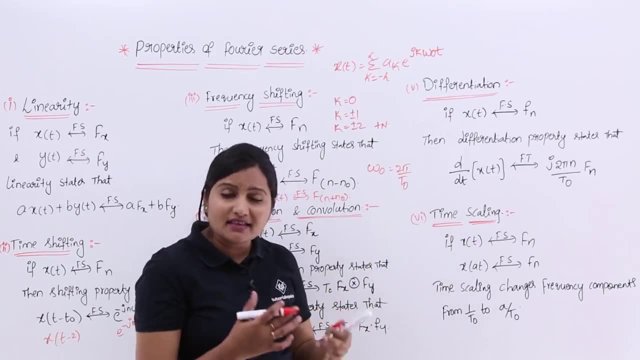 it will appear here. So actually omega naught is 2 pi by T naught, So but it will change 1 by T naught to a by T naught to a pi by T naught. like that it will change the frequency.